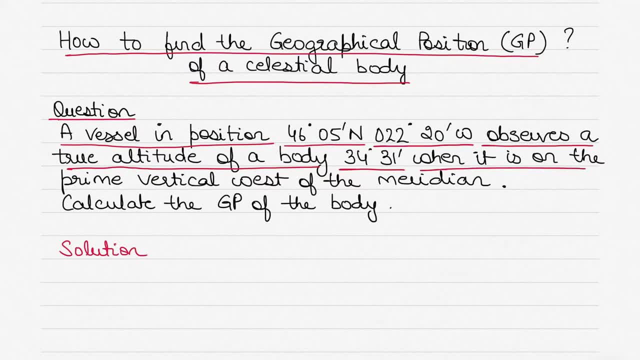 minutes and the true altitude was observed when it was exactly on the prime vertical west of the meridian. And the question says: calculate the gp of the body. Alright, so first I will explain to you what is gp and then I will show you how to. 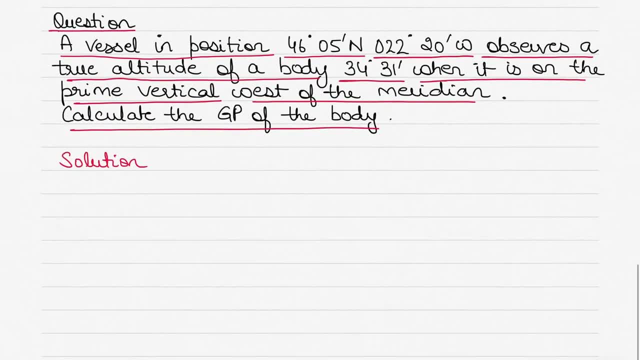 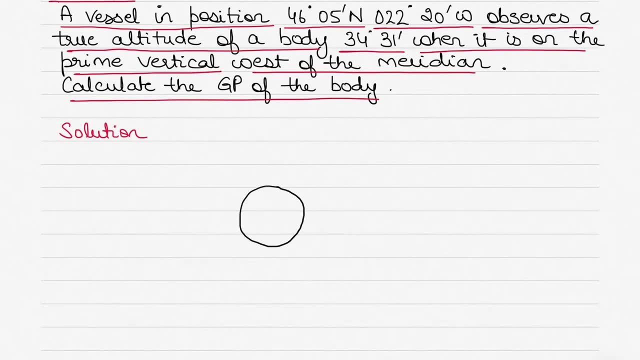 calculate the gp using the rational horizon diagram, or the p-z-x triangle, in this case, of course. Alright. so what is gp? gp is nothing but the geographical position of a celestial body. that means that if this is the earth, right, if this is the earth we project, the and a person is there on. 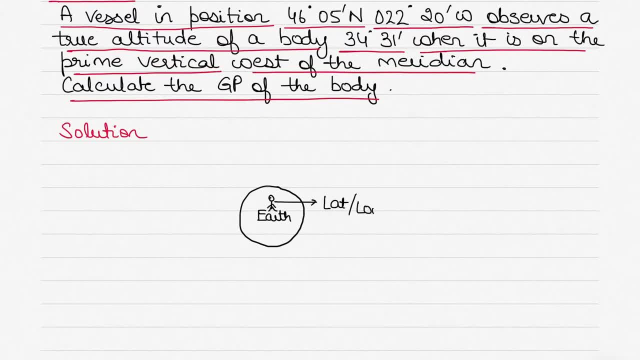 the earth. so the person's position is the position of the celestial body. So the person's position is on the earth, is known by his or her latitude and longitude. Right now, if we talk about a celestial sphere, a celestial sphere right, and we project this person onto the celestial sphere here, 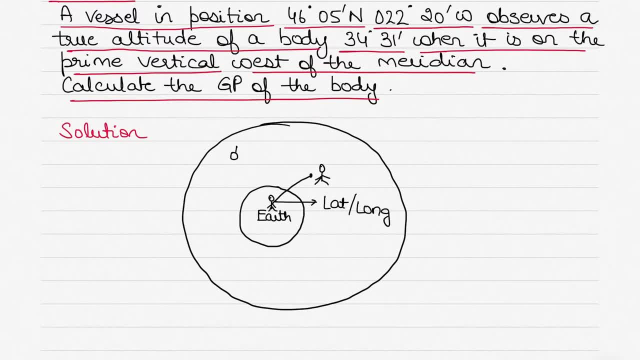 and we have a celestial body which could be the sun. This is my depiction of the sun. Now, the celestial body's position is not denoted by lat or long. it is not denoted by that. Alright, so what do we use? We use the declination of the body, Declination. 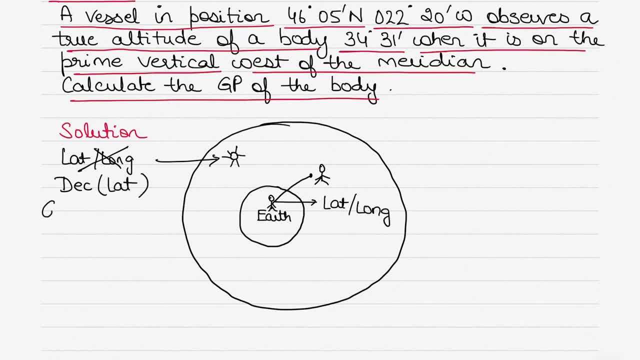 instead of lat, and we use the gha or the greenwich r angle instead of the longitude. So this is the all together. gha and declination make up the geographical position, or gp, of the body. Alright, so just like on the earth's position, our body is defined by the. 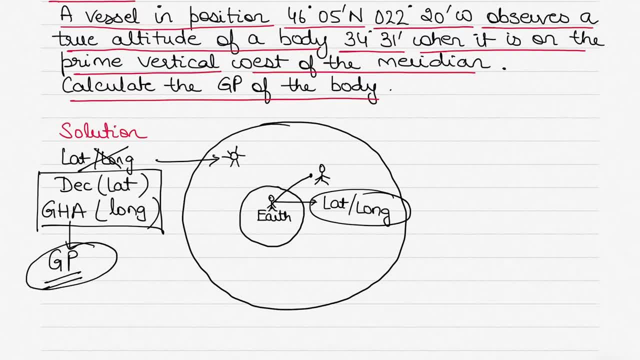 lat and long on the celestial sphere. it is defined by the geographical position, So that is gp. Now in this question, let's learn how to calculate the geographical position. if certain details are given to us, Especially if our vessel's position is given, how can we use that to calculate the? 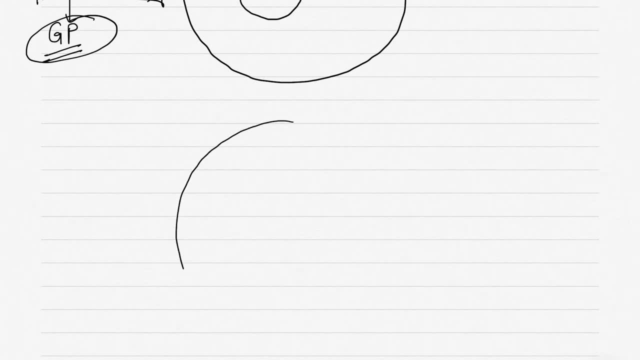 geographical position of a celestial body in the celestial sphere. To do that, I have to draw the rational horizon diagram again. Alright, now, of course, the circle. it should be a circle. This is not a perfect circle, But we make use of it. Then, this is the rational horizon, this is the celestial sphere. so we have. 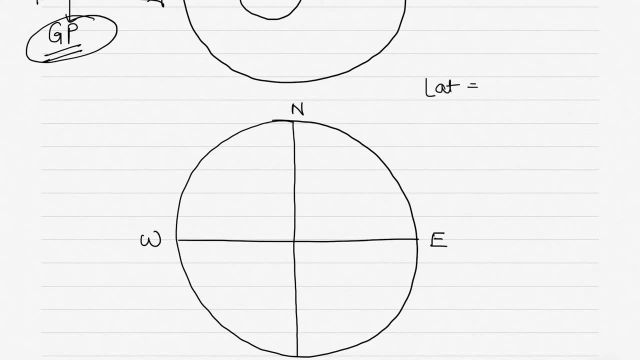 north, south and west east and then, because our latitude is 46 degrees and 5 minutes north, it is a north latitude. I will draw the north pole Here. the north pole is np, will be equal to the latitude right and then we draw the equinoctial. So the equinoctial has to be drawn. 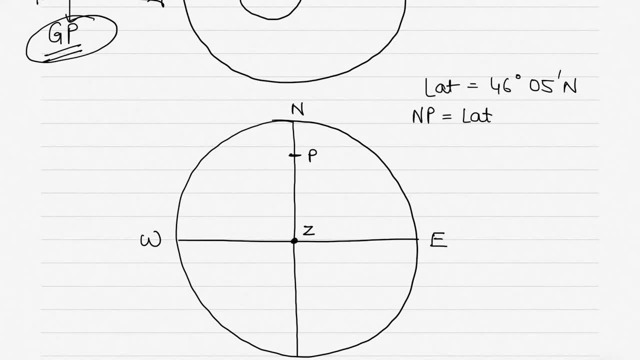 south of the observer. Now, where is observer? Observer is always in the center of the observer. This is the rational horizon diagram, Observer's zenith z, that is, u in the center of the rational horizon. So when I project the observer's position to the celestial sphere, that position is the 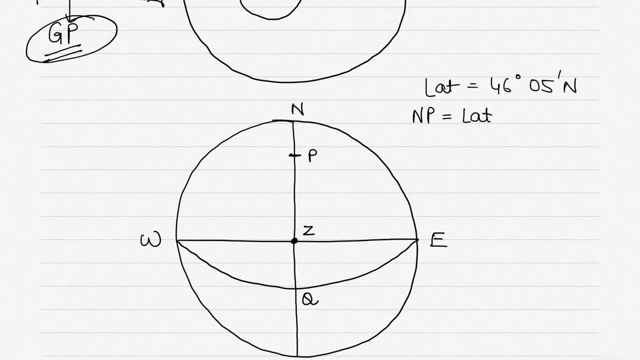 observer's zenith, And this equinoctial is wqe, q is the equinoctial, that is the celestial equator. Alright, and now you have the celestial equator, you have the observer. so here np will be equal to latitude, and also zq is equal to the latitude. 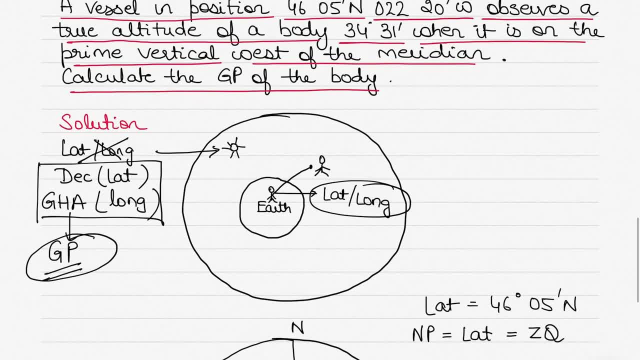 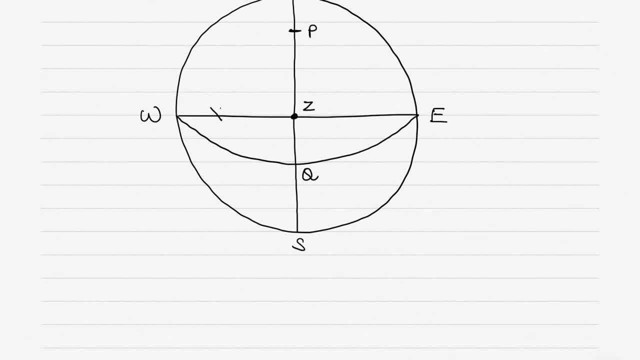 Alright, Now where is what else do we know? Now, we know the true altitude of a body, but we know that true altitude only when it is on the prime vertical west of the meridian. Alright, So prime vertical west of the meridian means somewhere here. Alright, So this is where, if it was east of 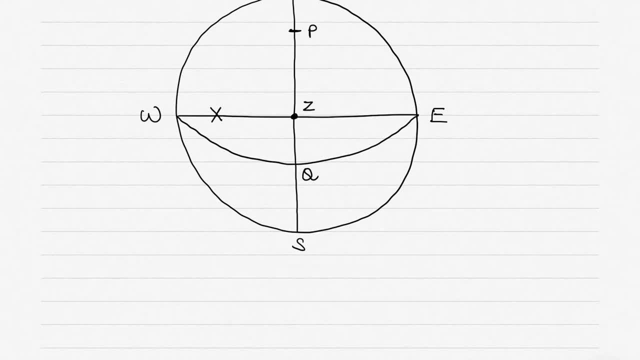 the meridian. I would have drawn this on the east side, but this is on the west of the meridian, Alright. So here we have found that that is where x is and that is the celestial body. And what do we know about the celestial body? is that we? 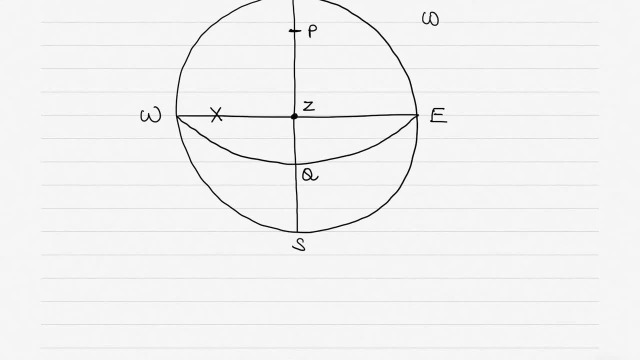 know it's true altitude, know what is the true altitude? The true altitude that will be w x. true altitude w x will be equal to what is given to us is 34 degree and 31 minutes, Am I right? So that is given to us and the question? and if we know that, then all we have to know is what is zx. 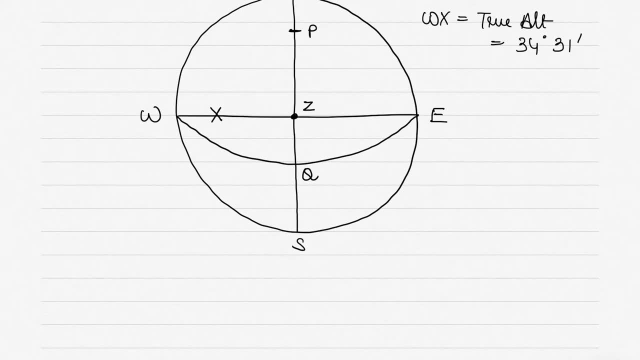 Now what is zx? zx is nothing but 93 Mari, 90 degrees minus the true altitude. now, why is it 90 degrees minus the true altitude? because every point on the celestial sphere is 90 degrees away from the observer zenith. all right now in this. 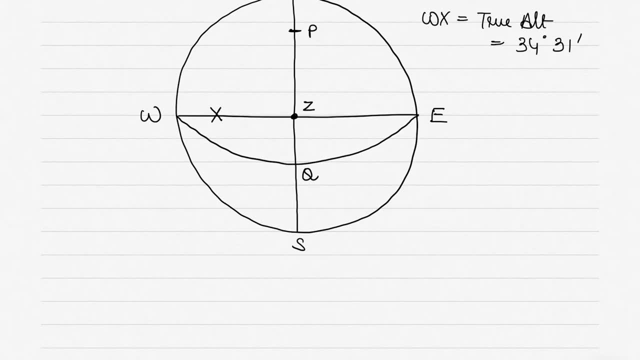 case, if you ask me what is prime vertical, then prime vertical is nothing, but it is a vertical circle passing through the east west points of the observer's rational horizon. so that is why i have drawn x there. i just thought i'll mention it just in case if you don't know, and then i will. 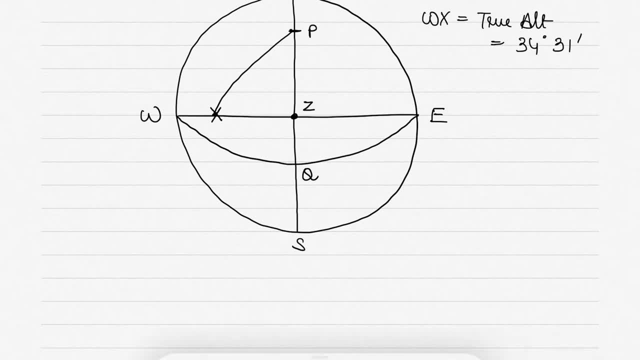 join pole to the equate, the celestial body. here now, of course, i will use a different color pen so that so wx here is 34 degrees, 31 minutes. each point on the rational horizon is 90 degrees from the observer zenith, so naturally zx becomes 90 degree minus true altitude, which in this case will be. 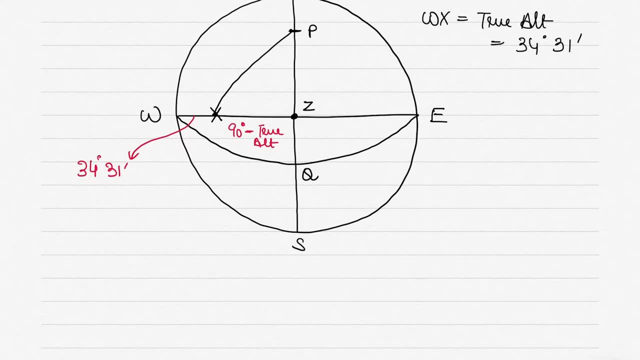 90 degrees minus 34 degrees, 31 minutes. so that would be, i think, 90 degrees minus 34 degrees and 31 minutes minutes. i work this question out together with you guys. so this is 55 degrees and 29 minutes. this is your zx, and i know pz as well. so how do i know pz? because i know np. correct, i know np. 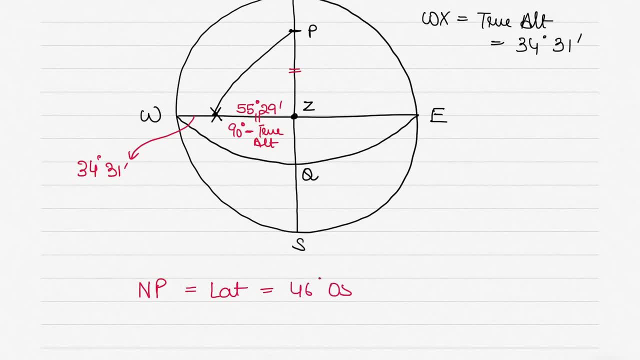 is equal to the latitude, which is equal to 46 degrees and 5 minutes. and i know that nz will be equal to 90 degrees because each point on the rational horizon is 90 degrees from the observer. so that is 90 degrees. so therefore, pz will be equal to 90 degrees, minus the latitude. 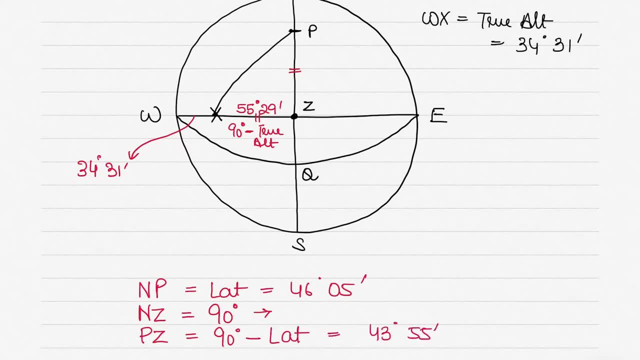 which in this case would be 43 degrees, 55 minutes. right, 90 minus latitude will be 43 degrees and 55 minutes. so i will call this 43 degrees and 55 minutes. now i know two sides. at least i need to know one angle, because i don't know any angles here. 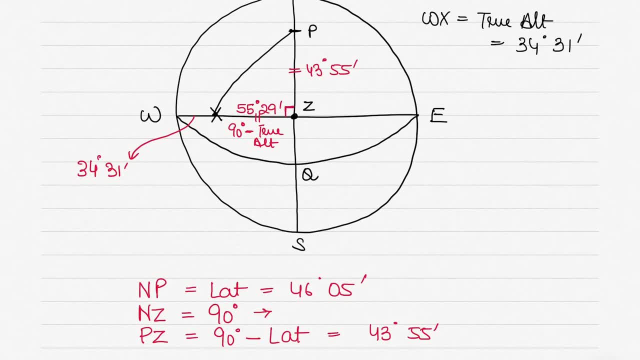 but i know that the celestial body is exactly west of the proporzionic, so that is 90 degrees and 55 minutes right, 90 minus latitude will be 63 degrees and 55 prime vertical angle z will become the 90 degree angle. so this will give us a right angle, spherical. 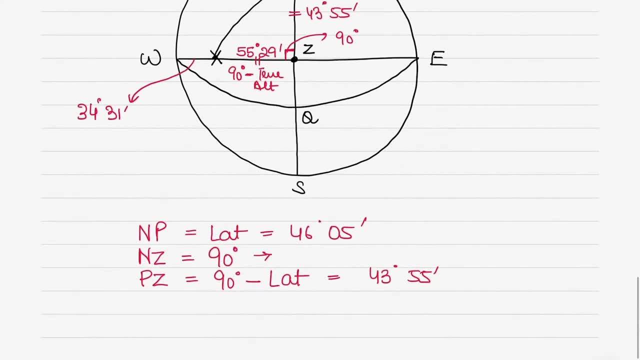 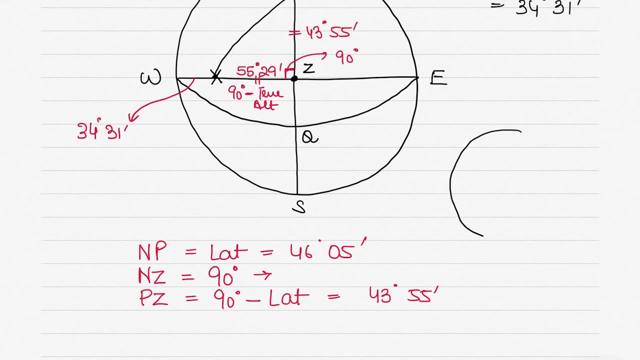 triangle which will help us to use the napier's rules. all right, so how do i use the napier's rules? if i, if i want to keep it on the same screen here, what will i do is i will draw another circle. so napier's rules. i am sure you have seen my videos on napier's rules. if you haven't, then 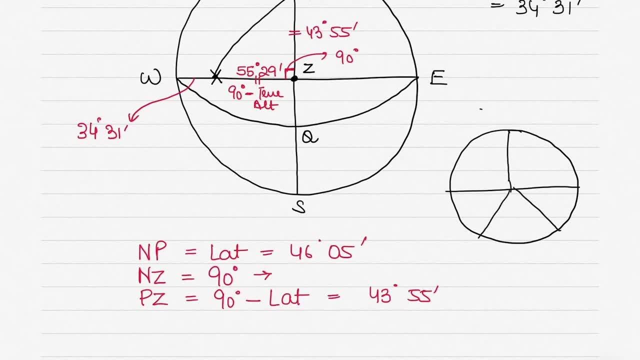 please go and watch my videos on napier's rules. i have explained it in detail. this is not the place i will explain it here, because then you know we are wasting time. so we have: z equals 90 degrees in angle in triangle p z x, p z x. triangle z is equal to 90 degrees. then we have p z. here we have. 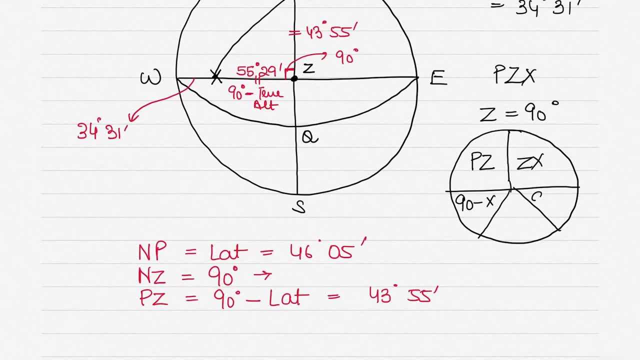 z x here, right, and then we have 90 minus x, 90 minus, sorry, 90 minus p. that would be 90 minus p and 90 minus x, and then 90 minus the remaining side. so we have p x. all right. now, p x is what we have to find, because we have to find the 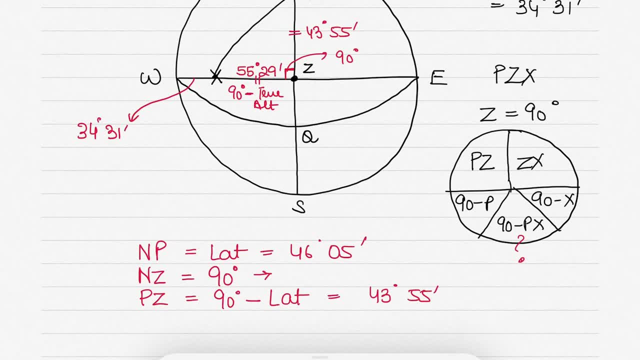 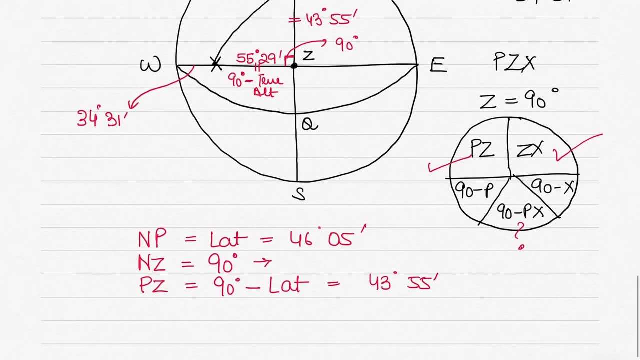 declination of the body. so we have to find p x, all right, and then i'll also show you how to find the g h. of course, that is where the longitude will come into play, all right, so we have p x here, and what do we know? we know p z and we know z x, all right. so then it's a simple matter of the. 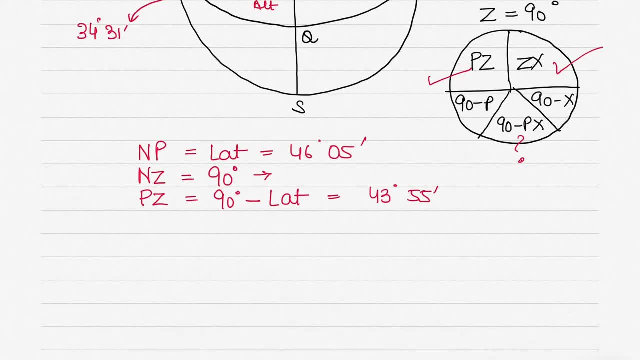 napier's rules. so how do i do that? so we have- i'll use a different color pen here, so we have- cos of the sine of the middle part, that is, sine of 90 minus p x equals cos of the opposites, cos of p, z and cos of z x. all right, so if you don't know the napier's rules, like i said before, please, 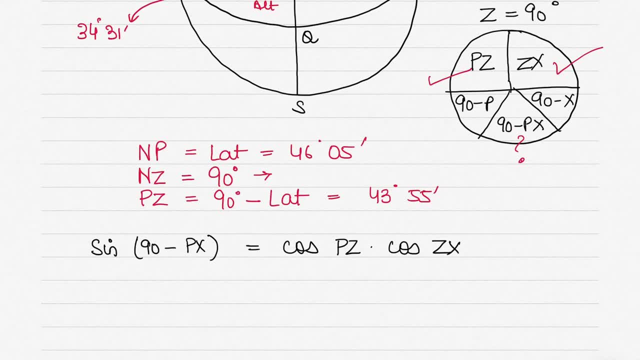 watch my other videos on napier's rules. i don't want to go into napier's rules here because that's a separate topic, so make sure that you watch those videos, all right. so what do we have here? so sine 90 minus p x. also. 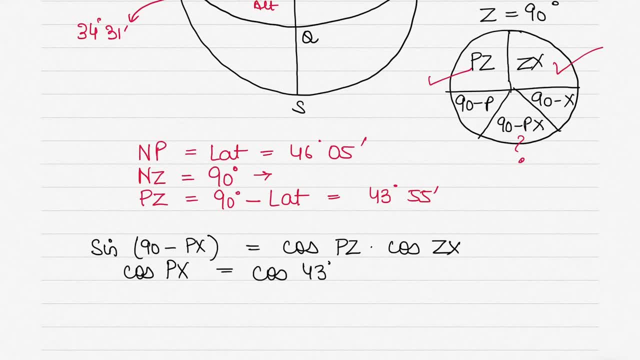 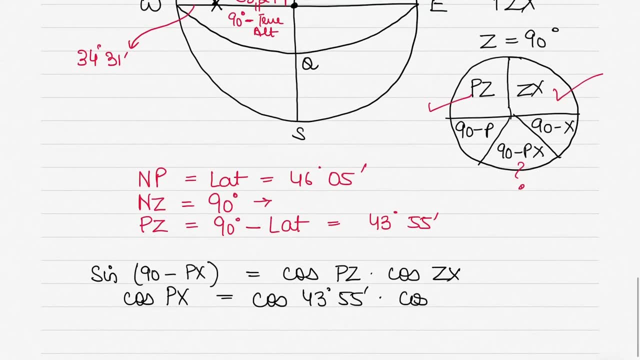 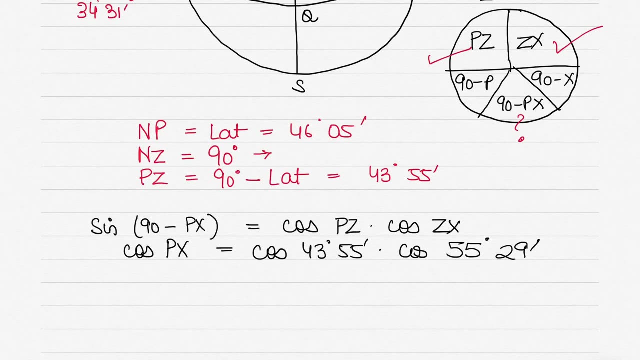 equals cos of p x, which i don't know, and cos of p z equals 43 degree, 55 minutes, and cos of z x equals, instead of z x, i write the value. so z x is 55 degrees, 29 minutes, all right, and then if i have to solve this, i will solve it together with you guys. 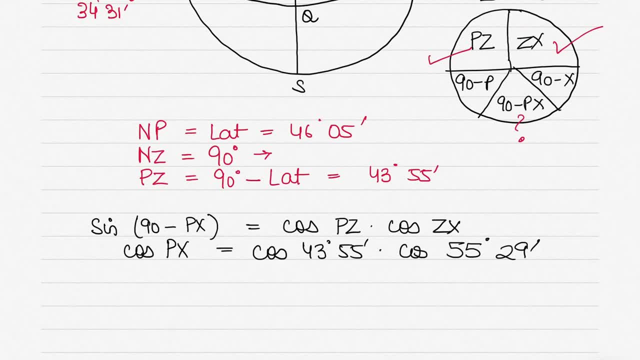 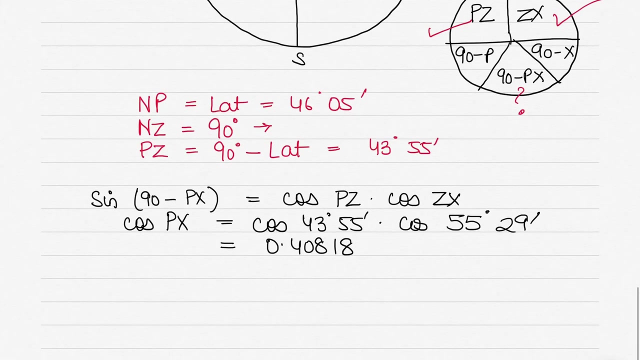 so we have cos of 43 degrees and 55 minutes multiplied by cos of 55 degrees and 29 minutes, and this will give me cos of p x equals 0.40818. so shift cos inverse. so so we have shift and cos inverse. so we have 65 degrees. so we have p x equals 65 degrees, 54.5 minutes. 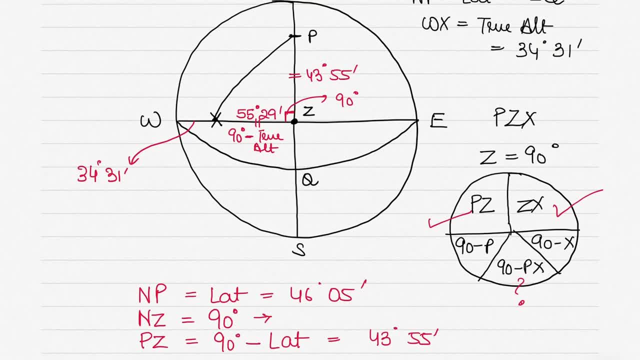 now, in this case, of course, p, x is the polar distance, so that is 90 minus. the 90 minus the polar distance will give me the declination right. so what will be declination? declination is always the angular distance from the equinoctial to the celestial body, so that is. 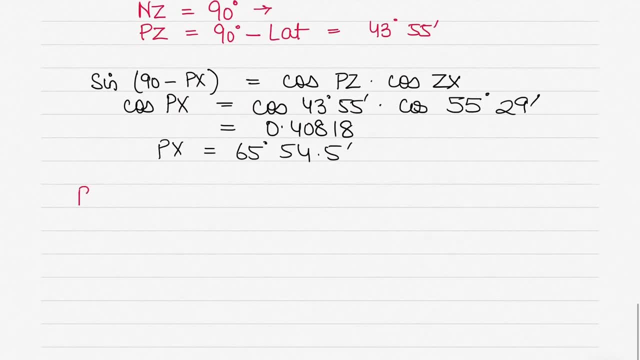 q x here. so q x is what i want. now i know p to q is 90 degrees, so p to q is 90 degrees, because from the celestial pole to the equator will be 90 degrees. so q x in this case would be 90 degrees minus p x. so we have 90 degrees minus 65 degrees. 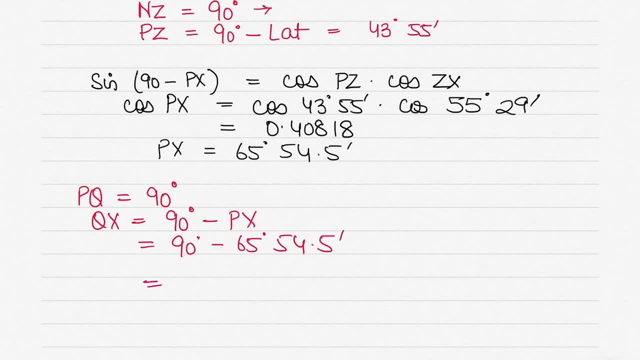 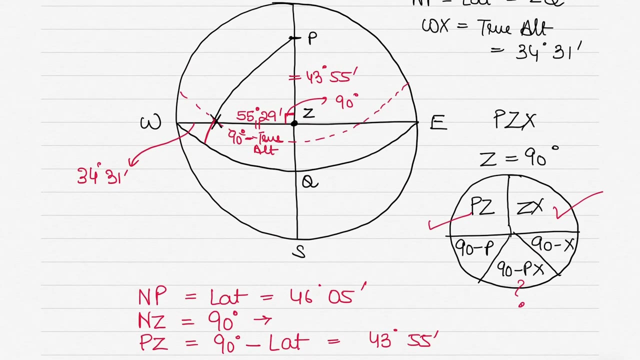 54.5 minutes, correct. so what do we have here? 24 degrees, 5.5 minutes. 24 degrees, 5.5 minutes, and is it north or south? now, what is q x? q x is nothing but the declination. remember that right declination is like latitude of the celestial body, so it is angular distance from the celestial. 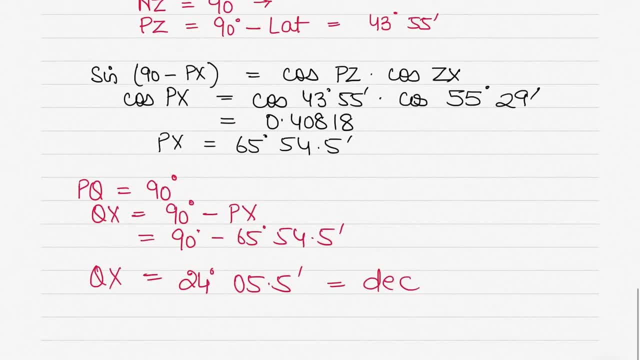 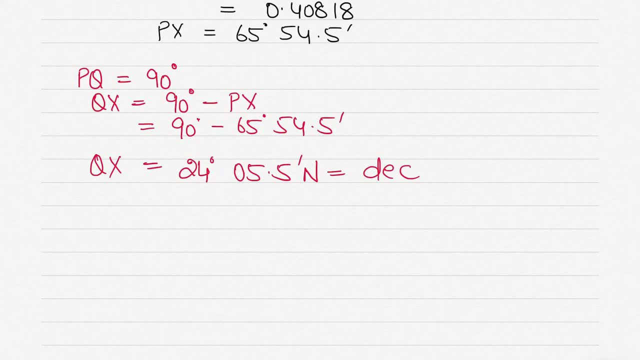 equator now, because x, X is north of the celestial equator. celestial equator is Q and X is north of it, so we will call it north, alright. So that is your declination. So one part is done of the geographical body. 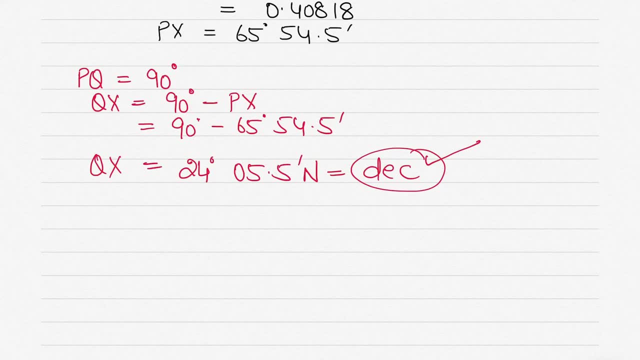 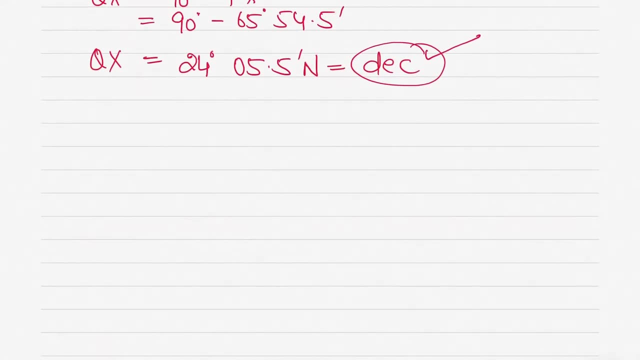 So I have found out the latitude, or the declination part of the geographical body. Now how do I find the GHA, or the longitude of the celestial body? So when I say GHA, we call it longitude, like I explained before, because on the celestial sphere we cannot have anything called longitude. 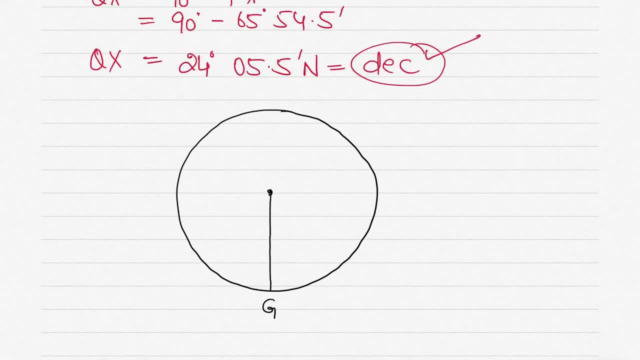 So what we have is the GHA. So what we say is that we have the Greenwich Meridian, G celestial Greenwich Meridian, and we know the longitude of the body. So I am here, somewhere here This is me, and what is my longitude? My longitude was 22 degrees, 20 minutes west, So 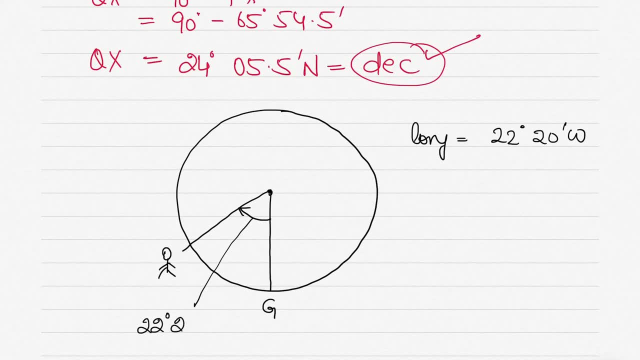 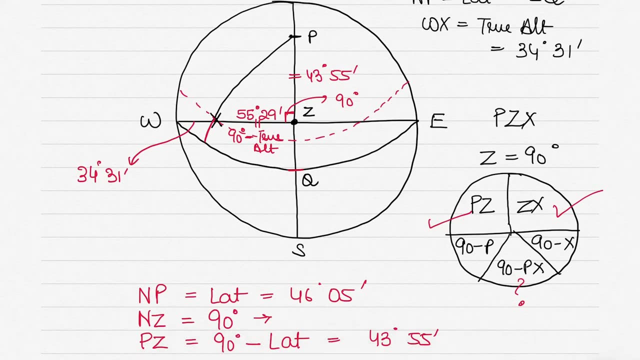 this angle here is 0.. 22 degrees, 20 minutes west. all right now, what else do I know? do I know my LHA? I know my LHA because, if I measure my, the angle, the or the bearing of the celestial body westerly from my, 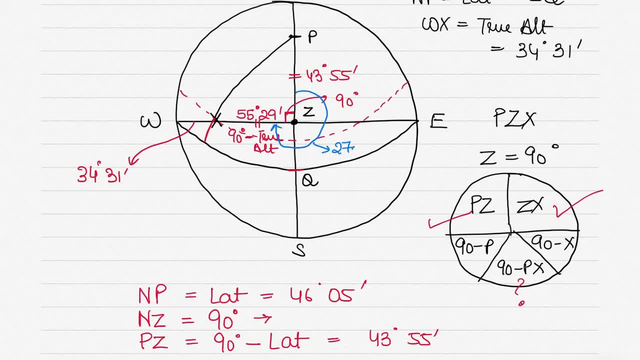 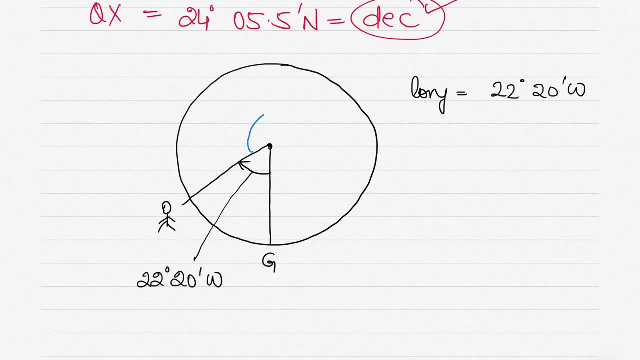 meridian to the observer's meridian. that will be about 270 degrees, because angle z is 90 degrees and the whole thing is 360. so I know that if I measure this angle here, this will give me my LHA. LHA is 270 degrees, right? so LHA is nothing but measured angle, measured westerly from the observer. 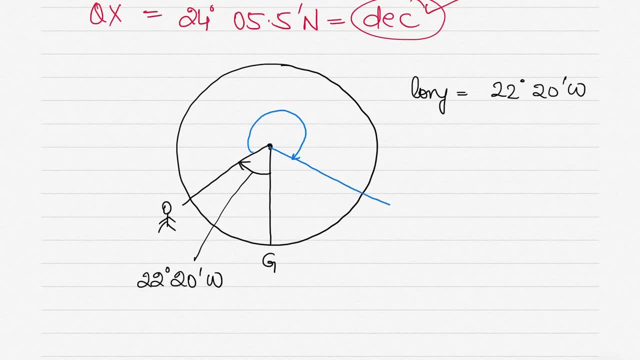 to the celestial body's meridian. this will be here, this will be x, or the celestial body right, and this angle here is 270 degrees. all right, so what is GHA now? GHA is nothing but angle, measured westerly from the observer to the celestial body's meridian. 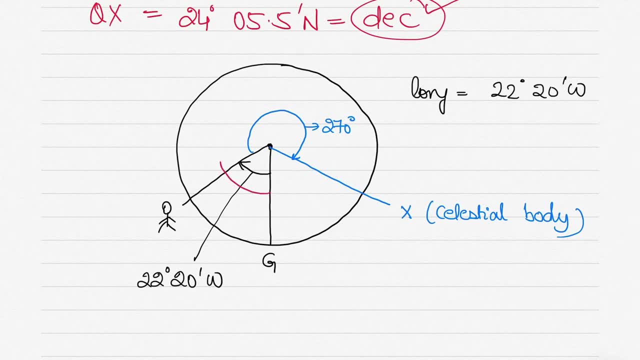 from the celestial greenwich meridian to the meridian of the celestial body. all right, so this is the GHA. this red angle is the GHA. all right, so how much is this? so, if you think about it, this is this: much is 22 degrees plus 270 degrees from there. 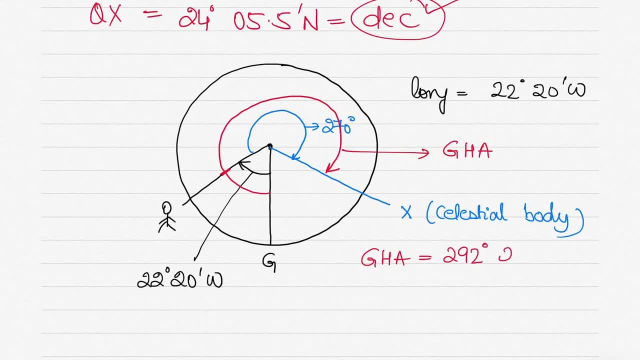 is, of course, 292 degrees, so GHA is equal to 292 degrees 20 minutes, correct, because GHA, as you can see, will be equal to. in this case, of course, it will be equal to longitude plus LHA, correct, as you can see? so we have 270 degrees plus 22 degrees 20 minutes. that's why, so I hope. 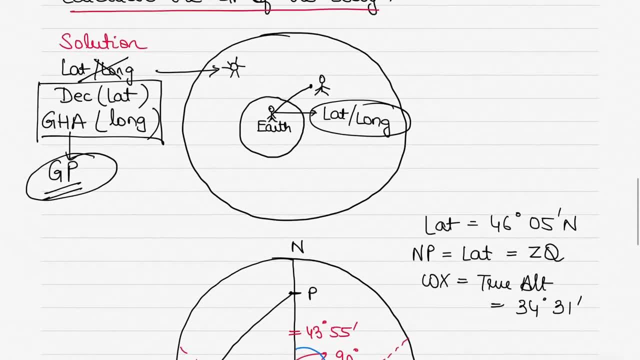 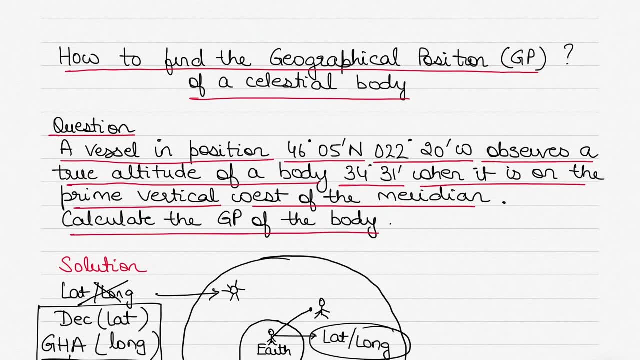 you understood this question correctly and there is no confusion regarding calculation of geographical position. if you still have questions or queries, feel free to contact me. write it in the comment section. I look forward to your feedback so that I can help my future videos. all the best, guys with the studies. study. 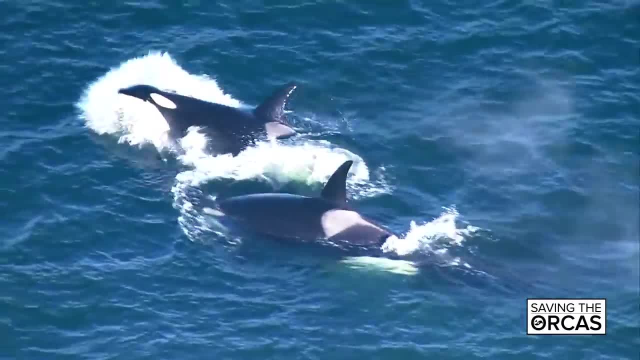 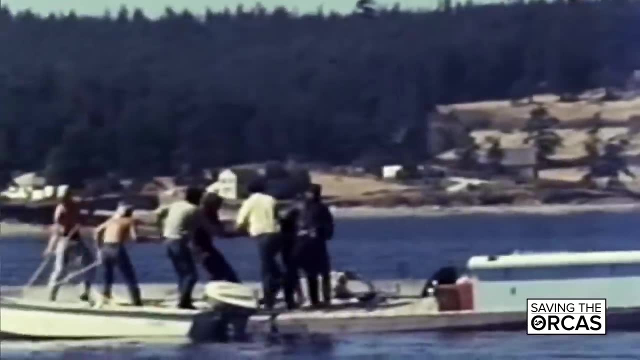 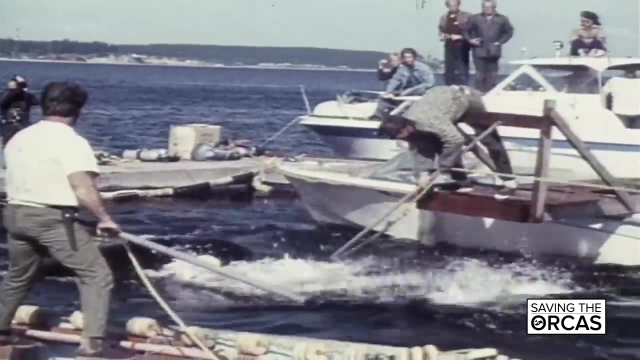 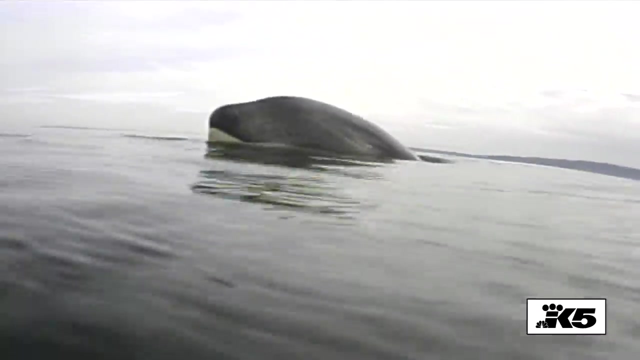 Orcas have been in an epic struggle to survive since the 1960s and 1970s, when they were captured and taken out of Puget Sound. Majestic whales ripped from their natural habitat and held in captivity at theme parks. Even after those captures stopped, the whales never recovered. 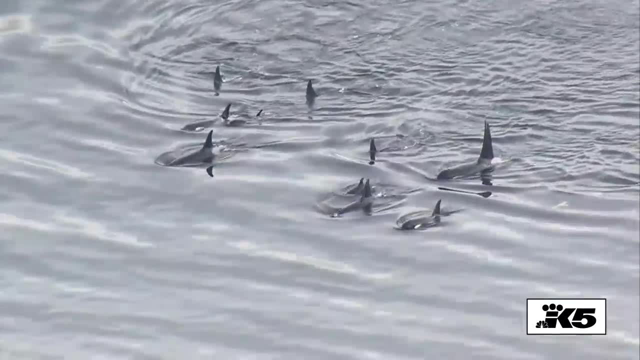 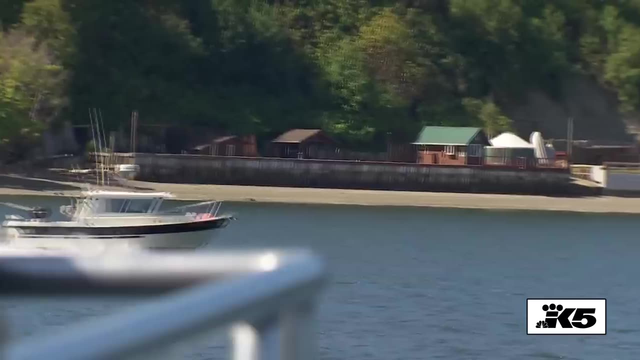 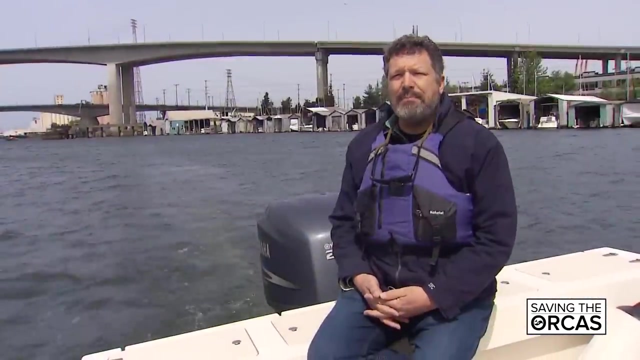 We don't have a minute to waste Now. the orcas left in the wild are facing new threats which could drive them to extinction. They need more salmon. Looks like a turbo. Their environment is killing them- Chemicals like PCBs, lead, copper and zinc. But there are. 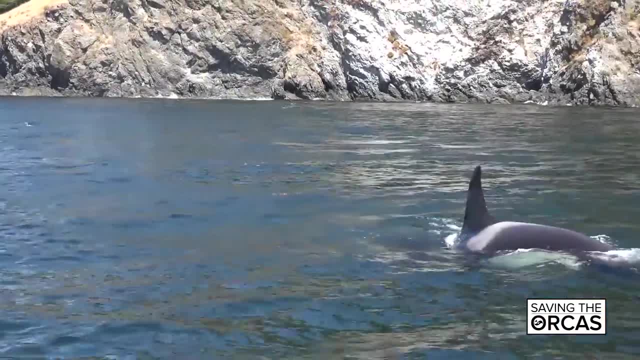 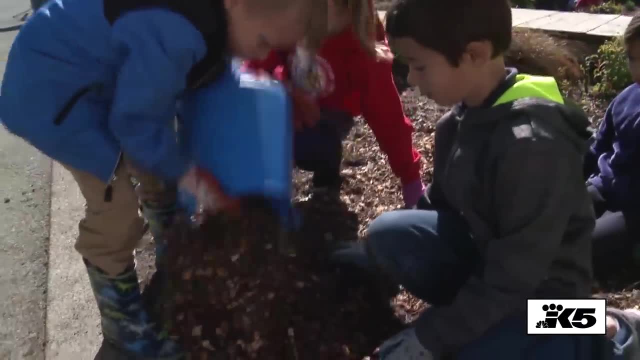 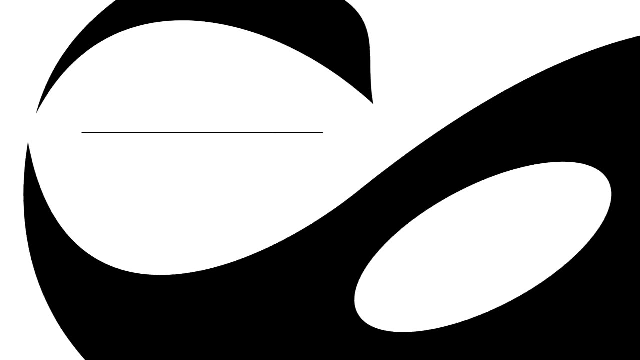 efforts to protect the whales. Efforts happening on the water- Easy thing to do to increase access to sea- Salmon has reduced noise- And on land. And why do we like rain gardens? Because they help orcas. Because they help orcas. This is a King 5 special report: Saving the Orcas. 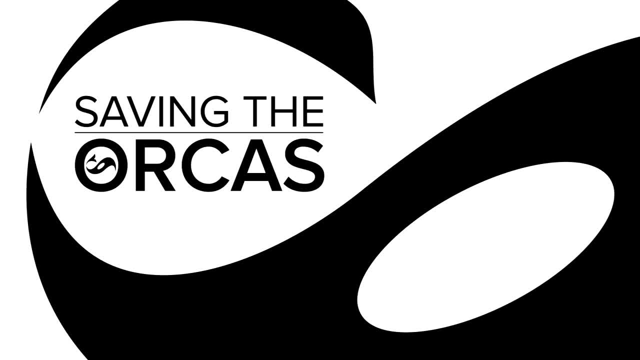 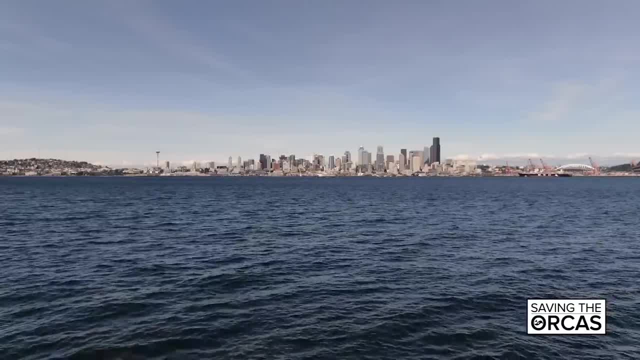 Here is your host King 5 environmental reporter Allison Morrow. We live in a very beautiful part of the world and we're some of the lucky few who get to see wild orcas right in our own backyard. For the next hour, we're going to learn about the challenges facing the southern 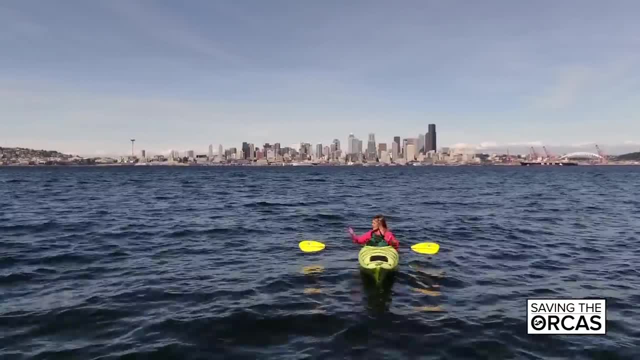 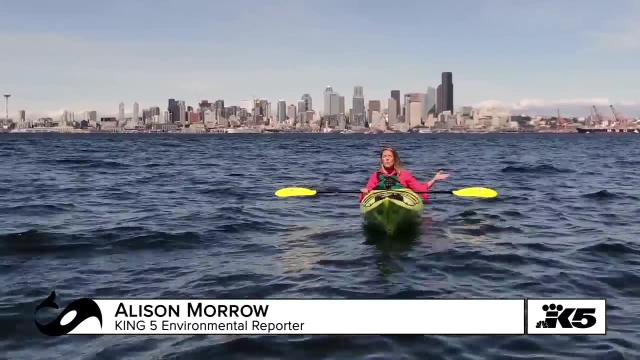 resident killer whales. They come here through Elliott Bay looking for Chinook salmon, their favorite food, But those salmon are also declining. Then there's all the boat noise and that makes it difficult for the whales to find the few fish that remain. And finally there's pollution in the water. 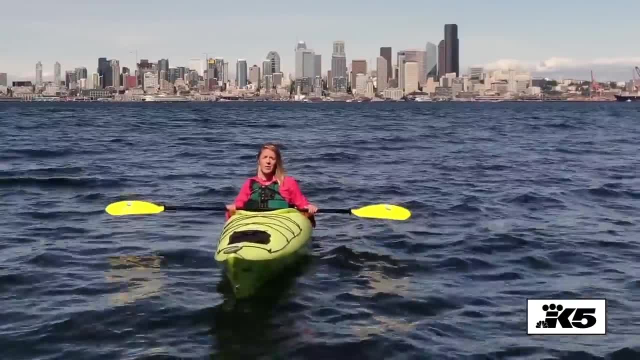 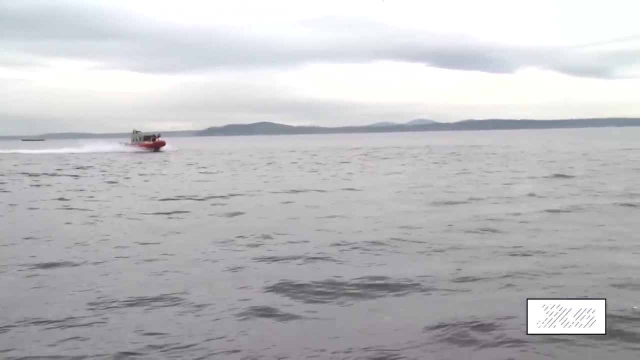 that's making the whales sick. With these very real challenges, it is possible we will see the southern resident killer whales disappear in our own lifetimes. The Salish Sea is like a water highway With all kinds of fish and animals. We're going to take a look at what's.